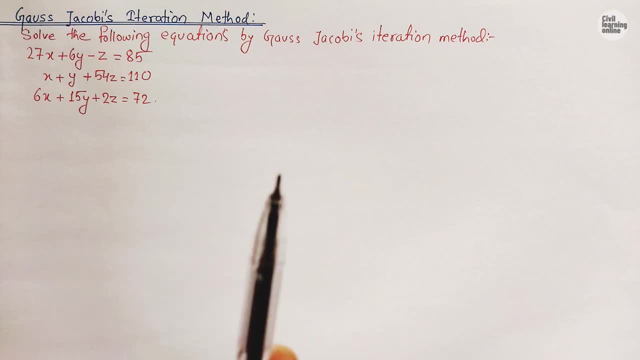 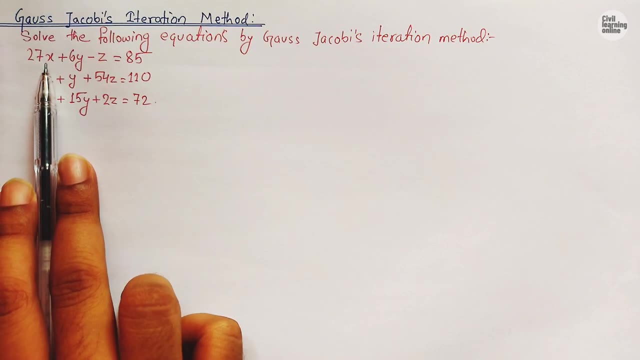 diagonal dominance property. what is diagonal dominance property? see, here, in the first row, we have the coefficient of x 27, or the magnitude of x 27, which is greatest of all, the. the sum of the coefficient of remaining two variables means 27 is greater than 6 plus 1. we i am not considering. 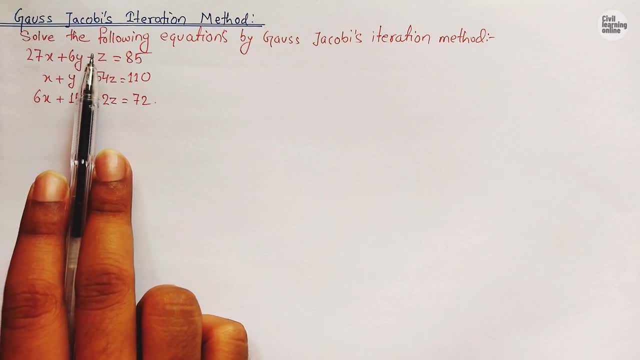 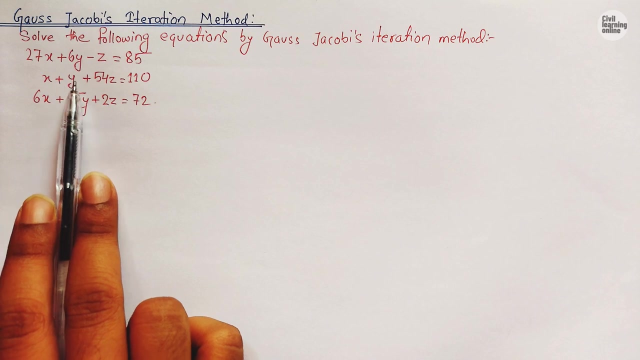 here the negative sign, because we we need to consider only the magnitude, means the how, what is how much coefficient it is carrying, disregarding the signs. so here we have 27: 27 is greater than 6 plus 1 it is greater, so it is okay. now in the second equation we have: 54 is greater than 1. 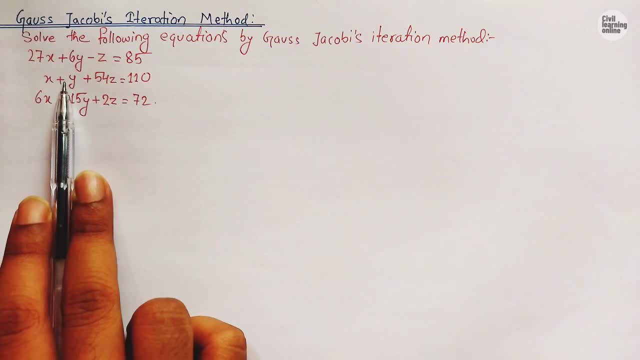 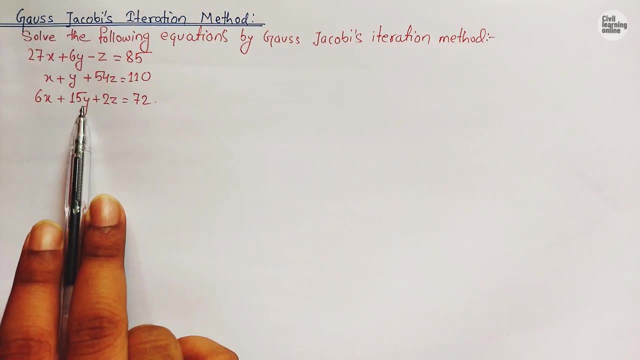 coefficient of x and coefficient of y, 54 is greater than 1 plus 1, 2, it is okay. similarly, coefficient of y. we have checked for coefficient of x, coefficient of z and coefficient of y. now for coefficient of y. coefficient of y, 15 is greater. 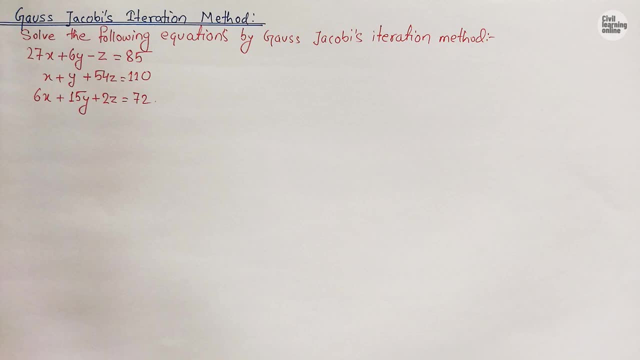 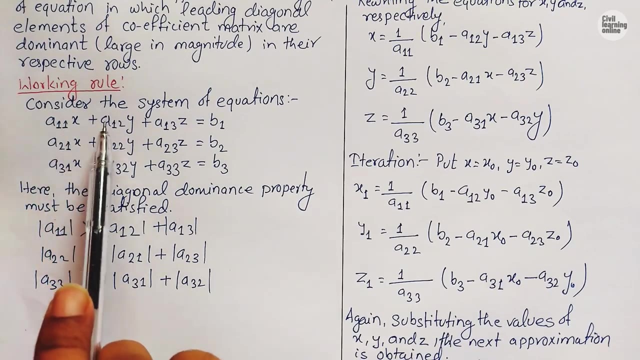 than 6 plus 2, 8. so here, if i have point out some points also, you can read it out by simply the pausing the video. see here we have working rule. this: a 1, 8, 1, 2, a 1, 3 represents the elements of. 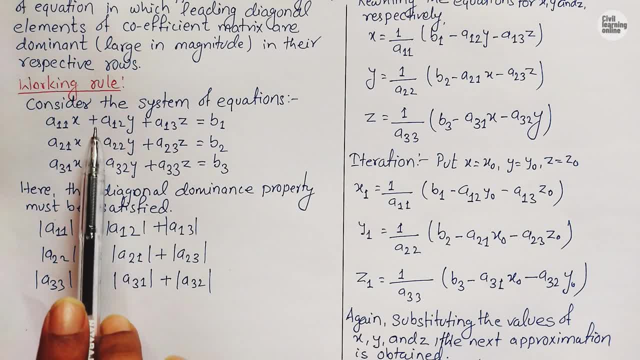 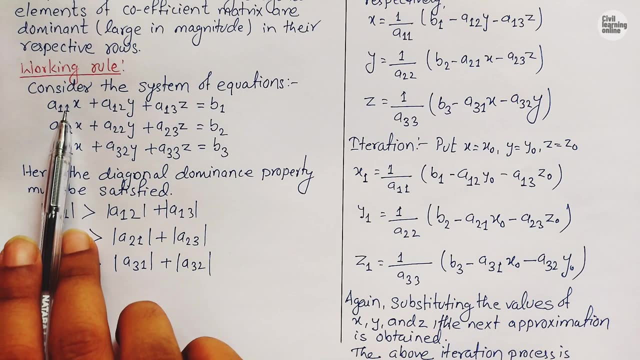 its raw or the coefficient of the different variables. similarly, we have a 2 1, a 2 2 a 2, 3 and if we are, we have the coefficient in this form. see here what we have: a 1- 1 means coefficient of first. 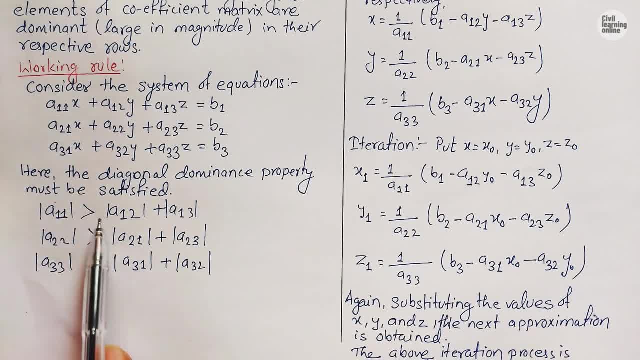 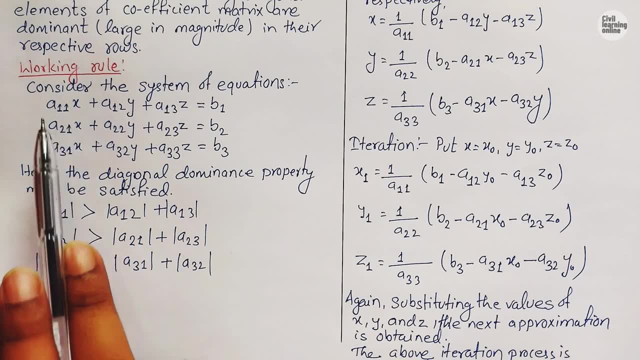 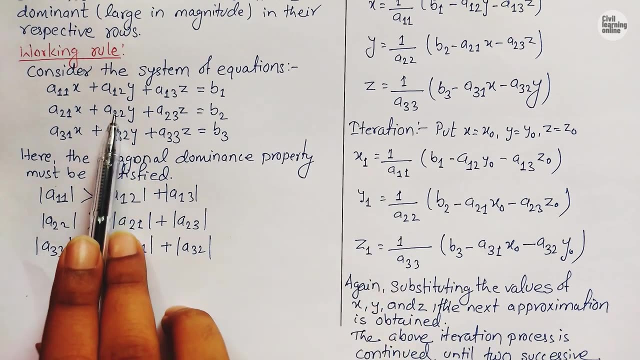 element, first row, first column, must be greater than the sum of the coefficient of other two variables, that is, a 1, 2, a 1, 3 sum must be less than a 1: 1. okay. similarly, we are not considering the sign here, simply adding the numbers. okay. similarly for a 2, 2 a 2 2 means coefficient of. 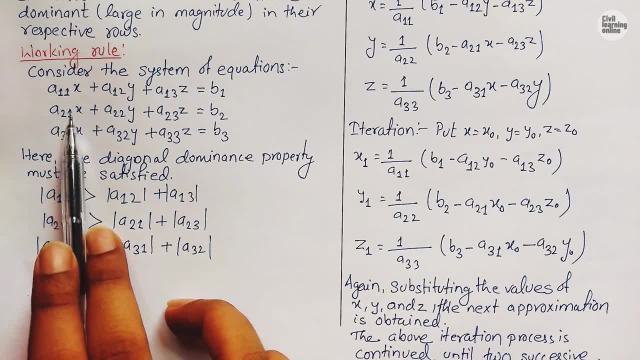 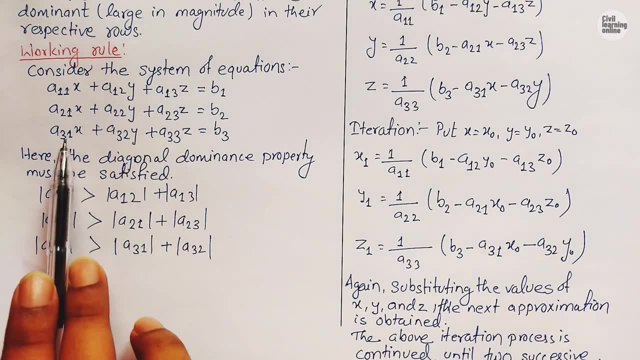 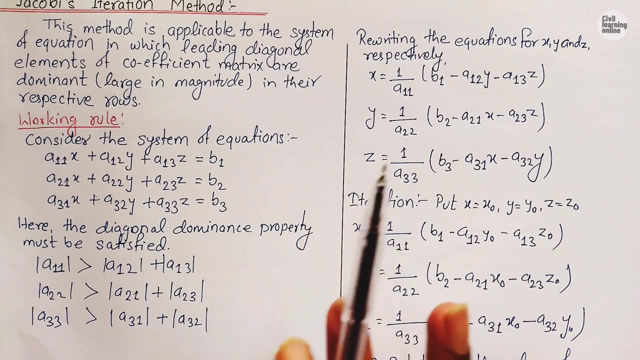 y must be greater than the coefficient of a. 2. 1 means a coefficient of x and coefficient of z in second row. similarly, in third row, the coefficient of z must be greater than the sum of coefficient of x and coefficient of y. now for working rule. if i am going to explain you the working rule further, then here, while after checking. 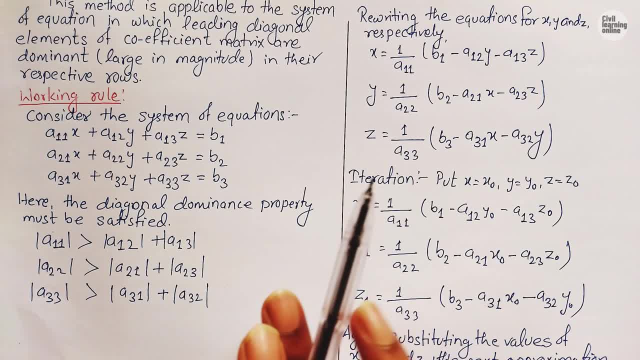 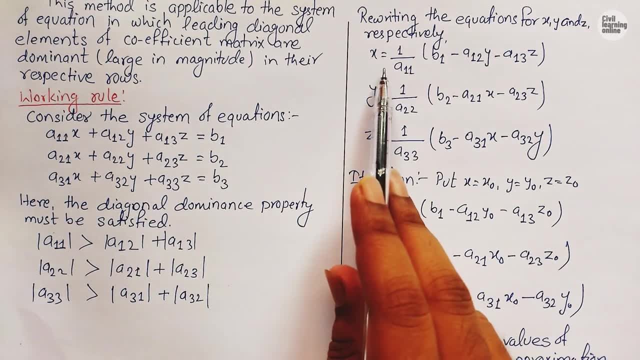 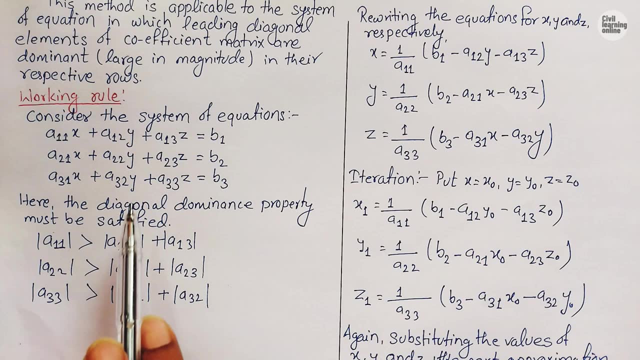 it. we do not need to show this while solving the numerical. it is just computed in our mind, which i already told you and i have shown you recently, uh, at the beginning of the video. now what we need to, we need to rewrite these equations in the form of x. i am going to explain it further in this numerical here and, for iteration, what we 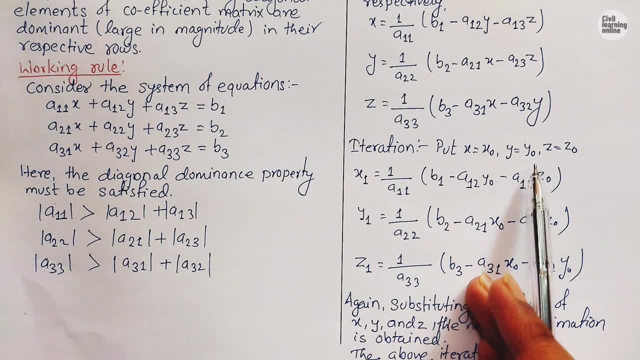 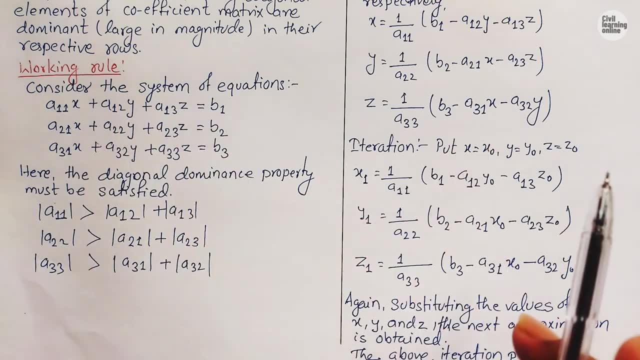 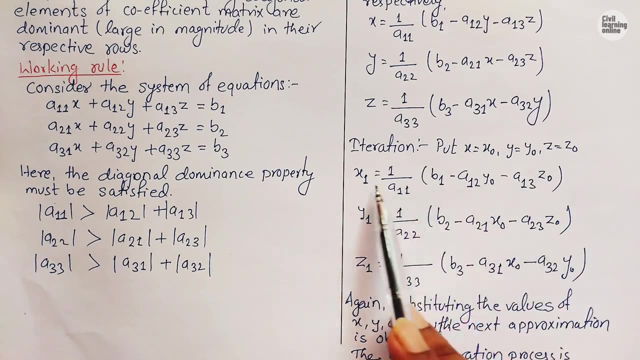 need to do is we have to proceed, taking x equals to 0, y equals to 0 and z equals to 0. okay, this is difference between the jacobi's iteration method and Gauss Seidel method. okay, uh, in the Gauss Seidel method, what we did, we took y note equals to 0, z note equals to 0 and put it: 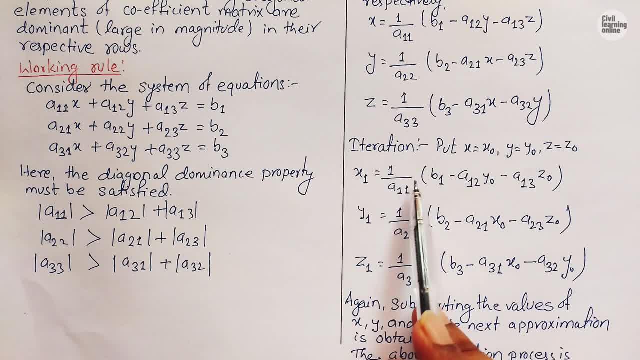 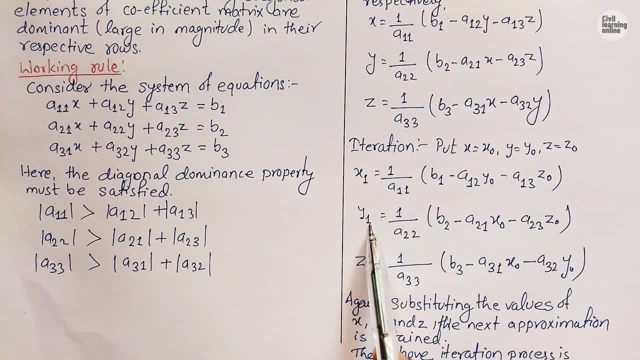 in the x okay for getting the value of x. and when we got the value of x, we use the recent value of x for in in equation for solving for y and after getting the value of x and y, we put that value for in while solving for z. but here what we need to do. 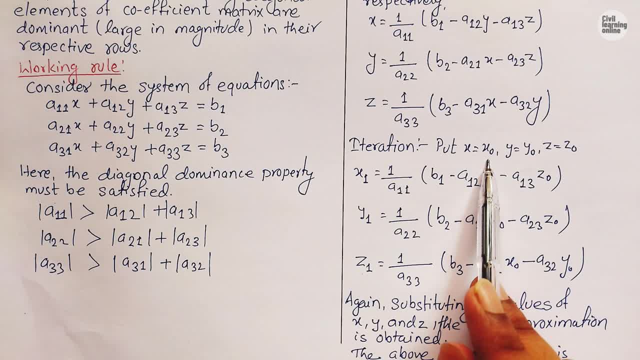 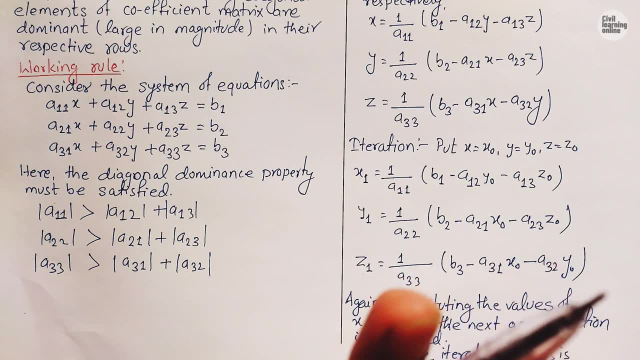 is we need to take all the initial value x naught, y naught, z naught equals to 0. if it is not given in the question means if initial value, initial iteration values are not given, then we will proceed taking x not equals to 0, y not equals to 0, z not equals to 0. now 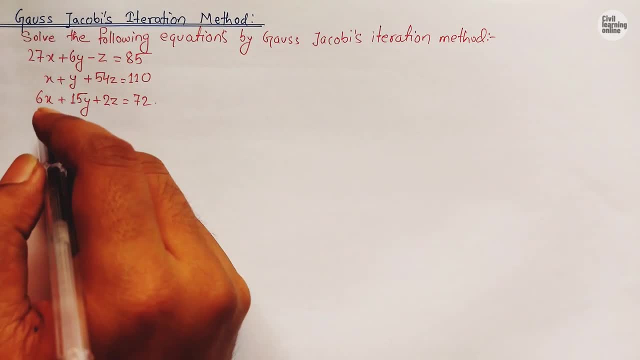 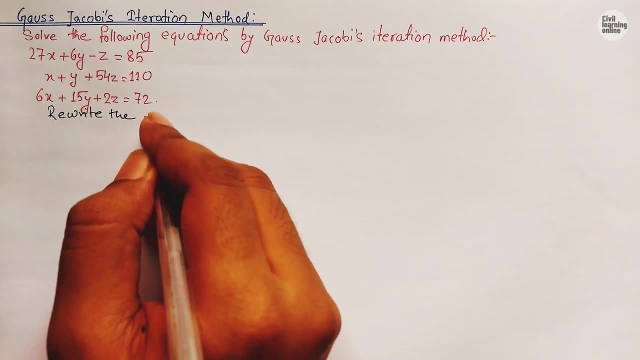 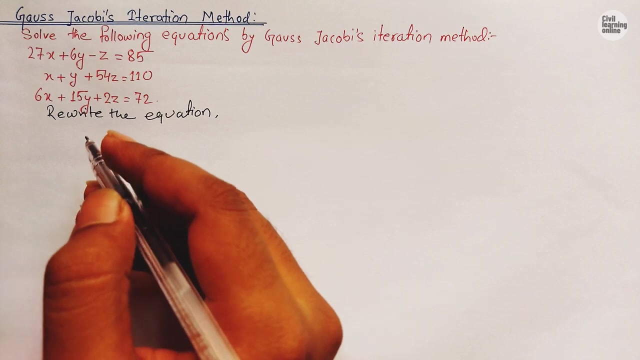 let us solve this problem further. so I am going to rewrite this, these equations here. so rewrite the equations, so rewrite the equation. what we need to do is we have to- ah, write it accordingly means the in first, first, first equation, coefficient of x must be greater, greater than or equal to 0. 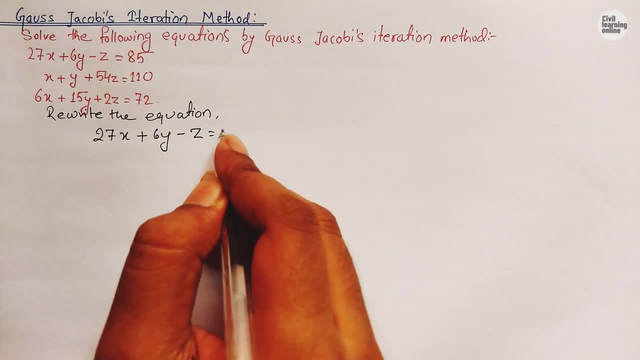 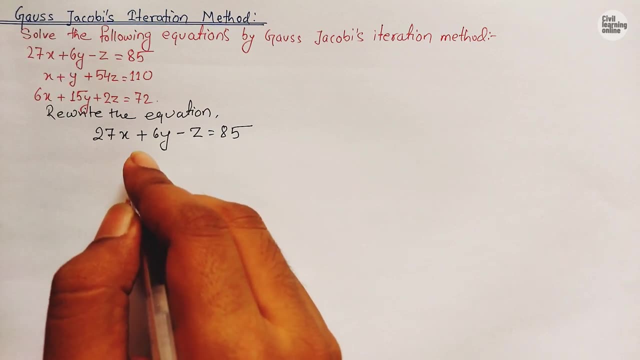 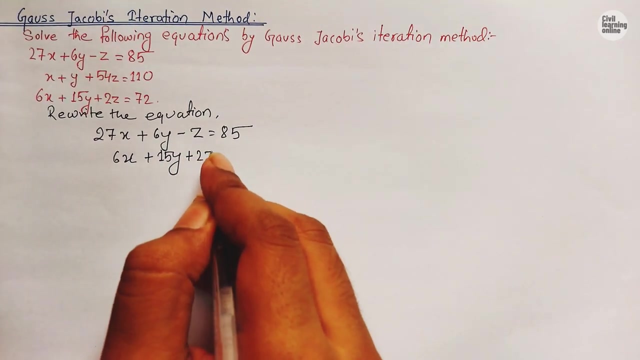 let us write the latest: z equals to 85. similarly, we have to interchange these two equations so that ah in the in second equation, coefficient of y will be greater than other two variables: 6 x plus 15, y plus 2 z equals to 72. similarly, we have x plus y plus 54, z equals to 110. now 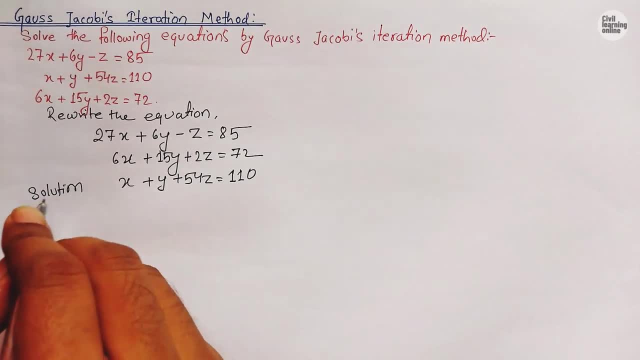 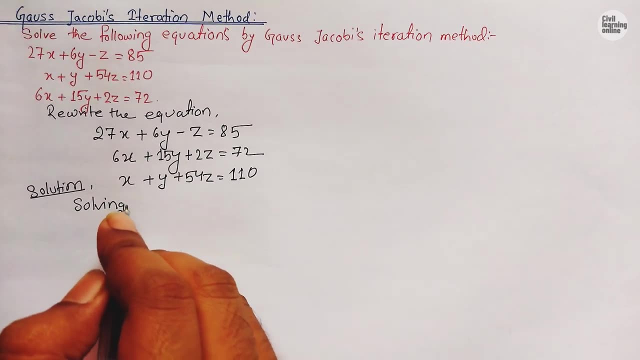 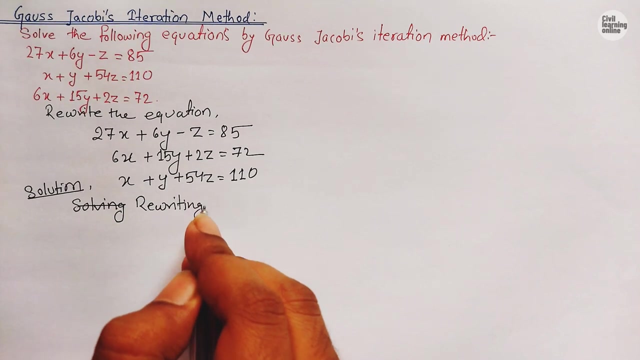 we have to 1, and then when I was writing that we can put seventie 0, 1 something in places, we are there, so again we have to put and it means it will be greater than 0 for now. so if andar, two characters between the two terminals, so will also be. 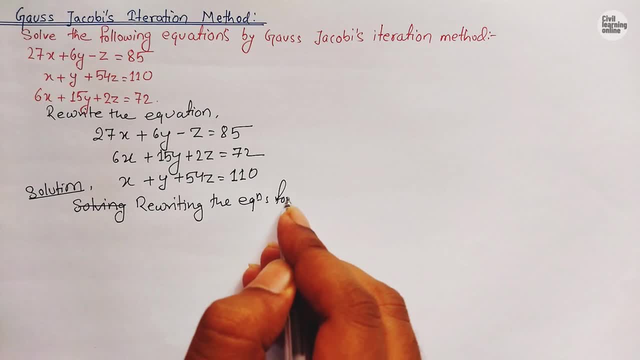 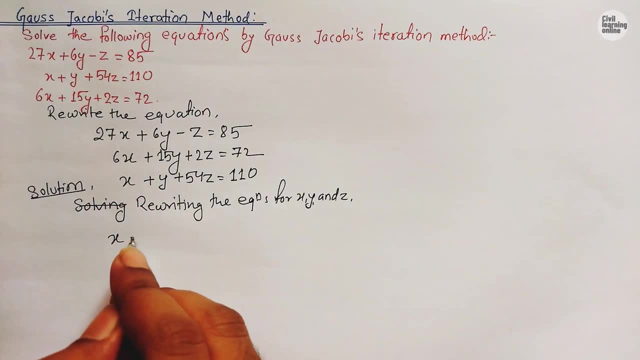 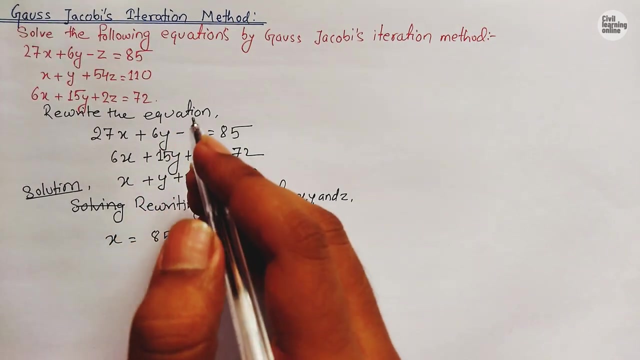 greater than 0. so y equals zero. small x times y equal to 1, or it is not meant or it is not exactly equal. that for short. so this will be equal to it will be nothing, but rather we will have here 85 minus 6y. just bring the other terms to other side of equals to means. 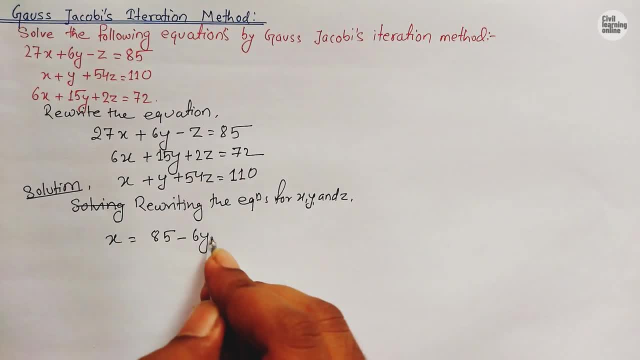 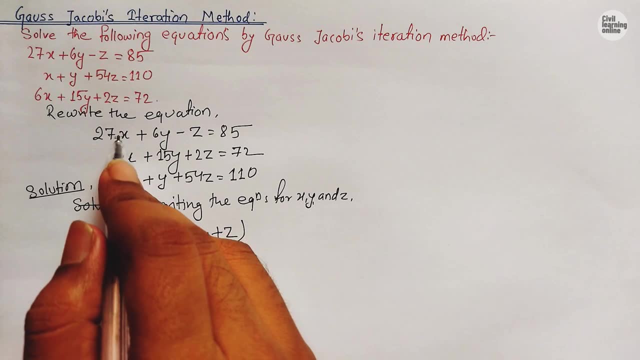 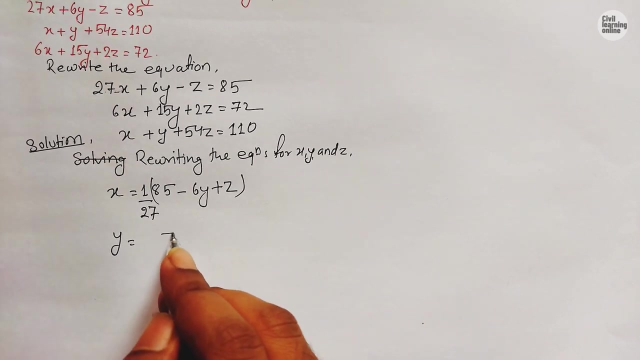 here 6y is positive, so it will be minus 6y and z is negative, so plus z. and this whole divide by 27 means here the 7 is 27 multiple with x, so I have divided this. similarly for y, we will have here 72 minus 6x, minus 2z, and this whole divide by 15. similarly for z, we 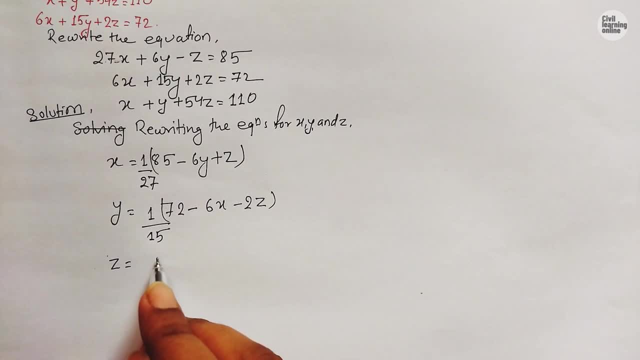 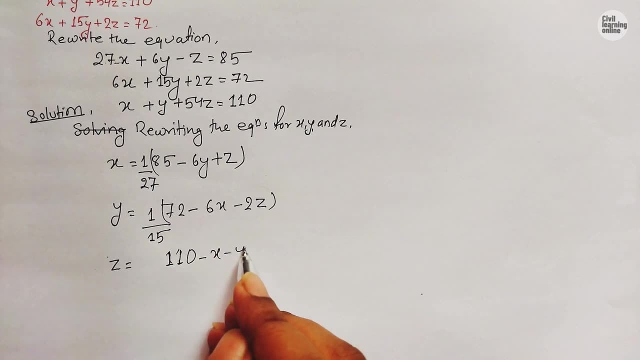 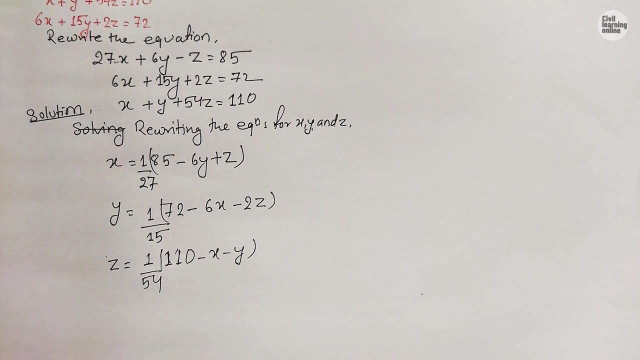 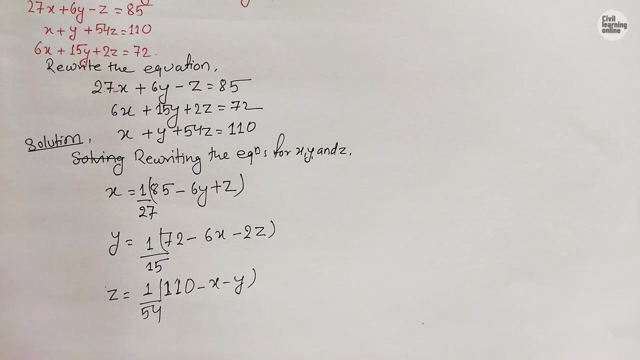 will have here: z equals to 110, 110 minus x minus y, and this divide by 54. okay, now we will proceed. the initial first iteration and the first iteration we will take: x not equals to 0, y not equals to 0 and z not equals to 0. so I 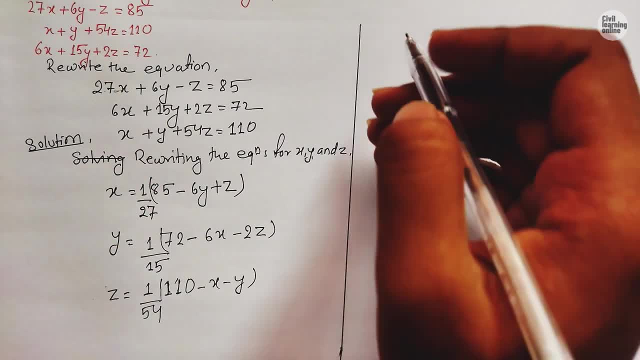 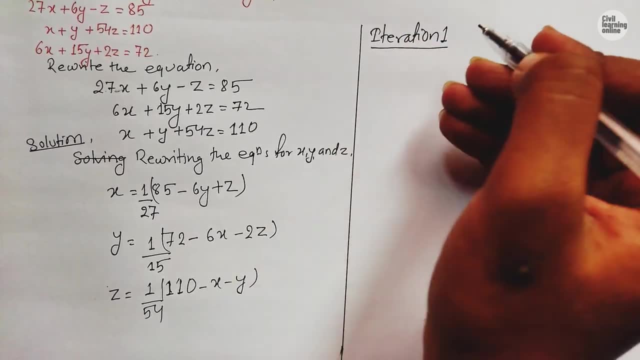 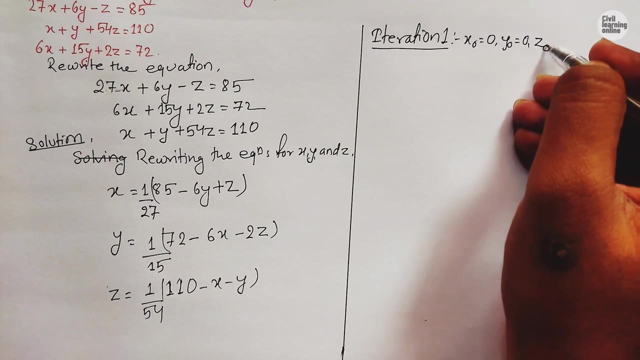 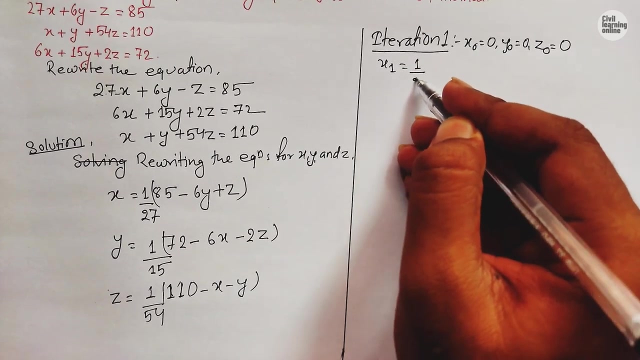 am going to write here. use this portion for iterations. so we have iteration 1.. For iteration 1 we will take x not equals to 0, y0 equals to 0 and z0 equals to 0. so here we will do: x1 equals to 1 by 27 times. 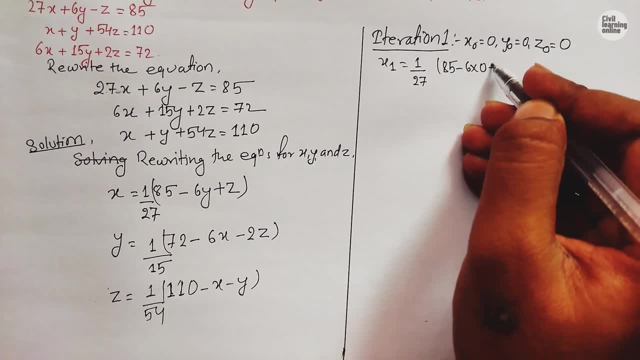 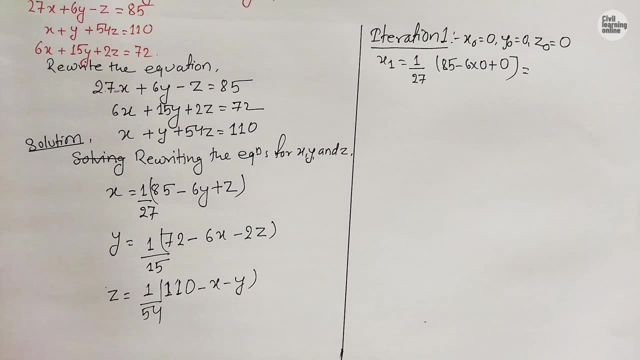 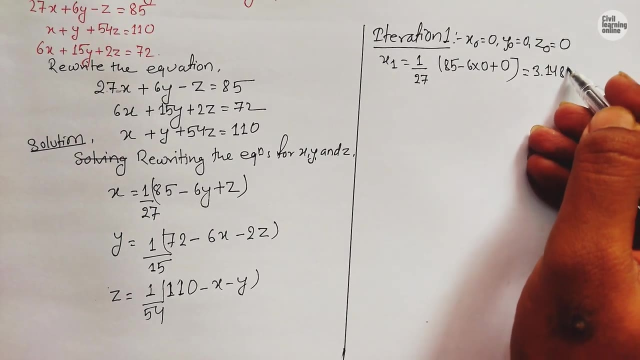 85 minus 6 times 0, plus z. in place of z we will put it 0. so on solving this, we will get the value of x1 equals to 3.1481. you can take it up to 3 decimal place or 4 decimal place. 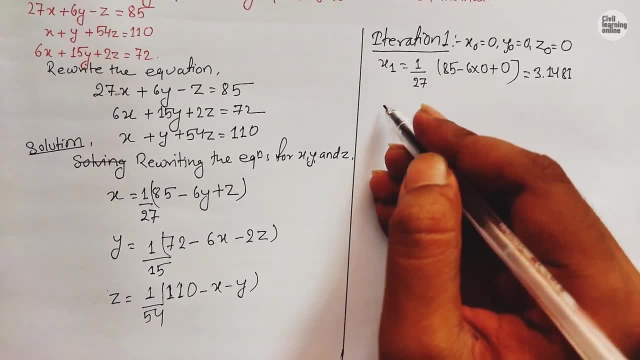 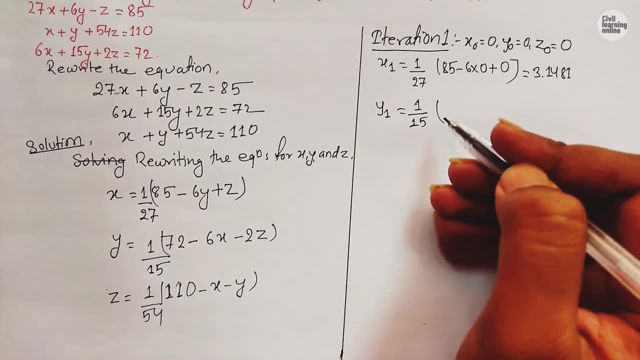 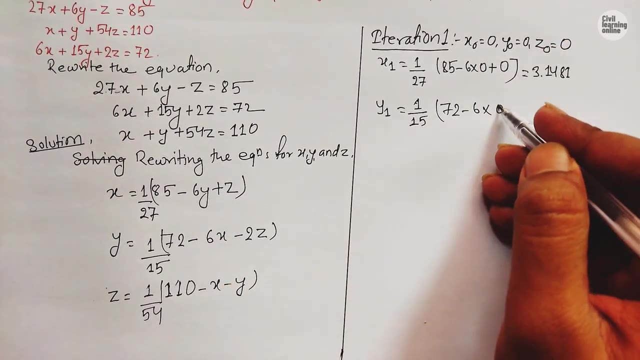 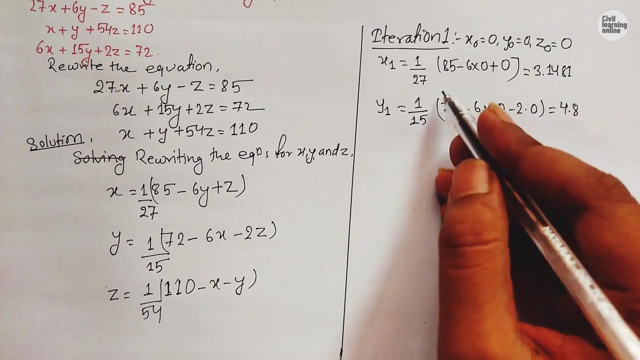 it is up to you if not mention in the problem in the question. so in y1 for y1, we will take 1 upon 15 times 72 minus 6 times. in place of x we will put 0, 0, 0, 2 times z. so i hope you are. you might have noticed the differences in gauss-seidel. what? 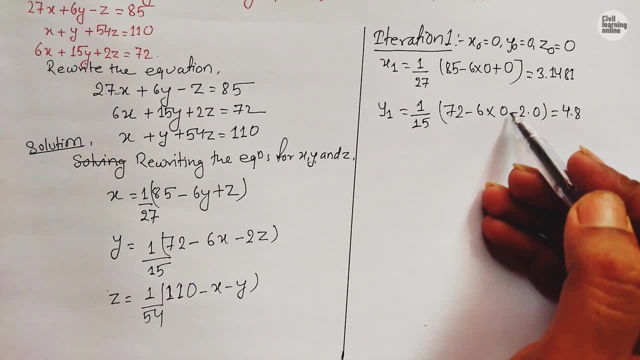 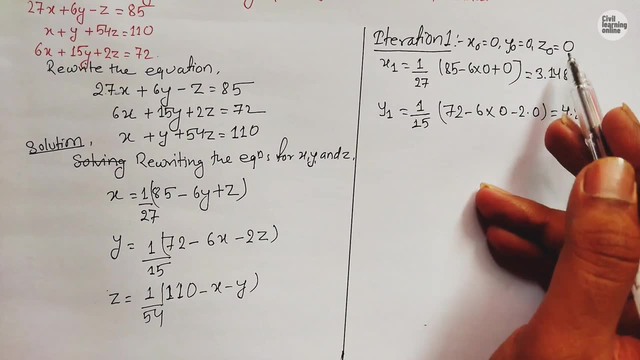 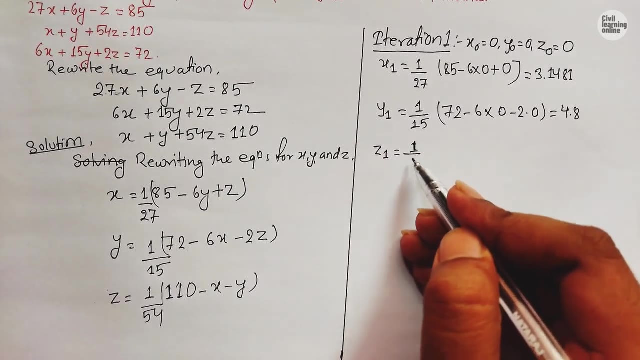 we have done we. why what we would have done is, in place of x, we will would have used this value, but in jacobi's iteration method we will take this: x0 equals to 0, y0 equals to 0 and z0 equals to 0. so again, z1 equals to 1 upon 1 upon 54 times 110 minus. 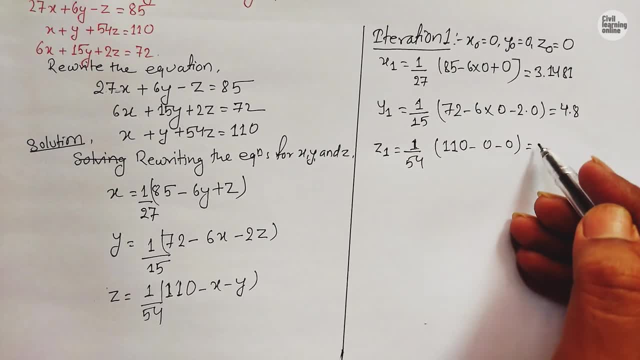 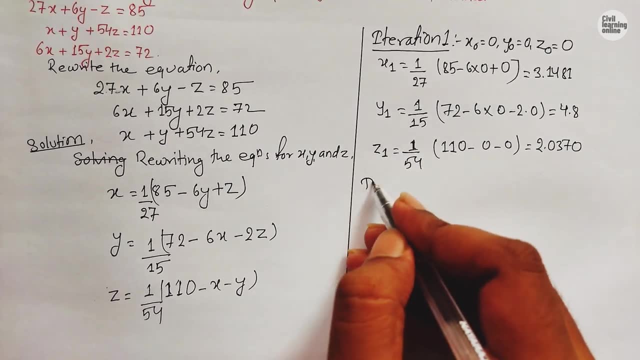 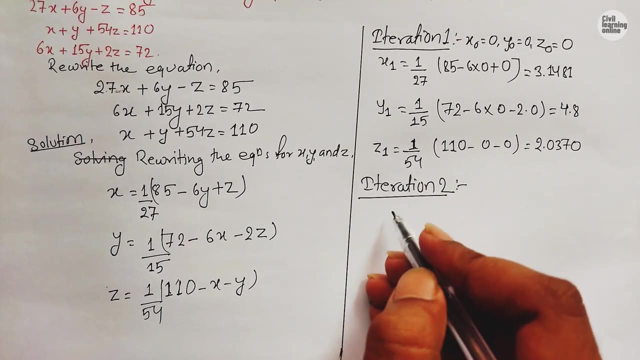 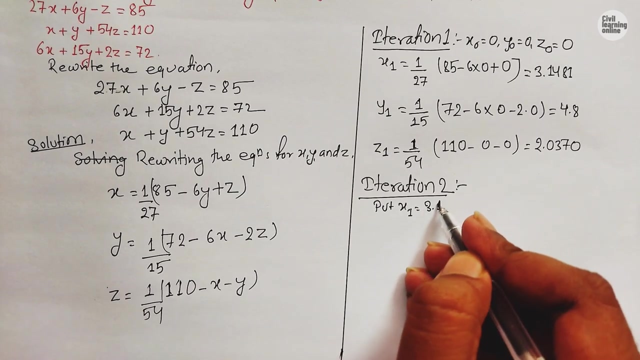 0 minus 0. on solving this, we will get the value of z1 equals to 2.0370. ok, now for iteration 2. for iteration 2, we have we need to put. we need to put: put: x1 equals to 3.1481, y1 equals to 4.8. 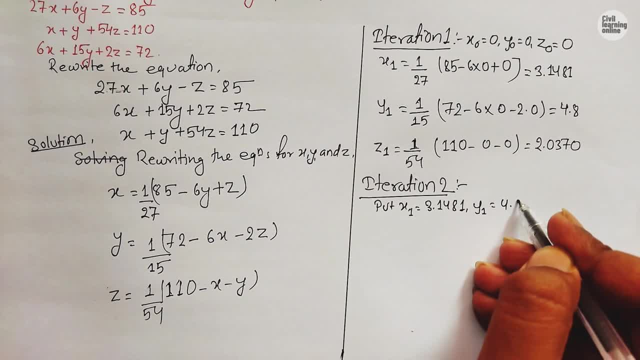 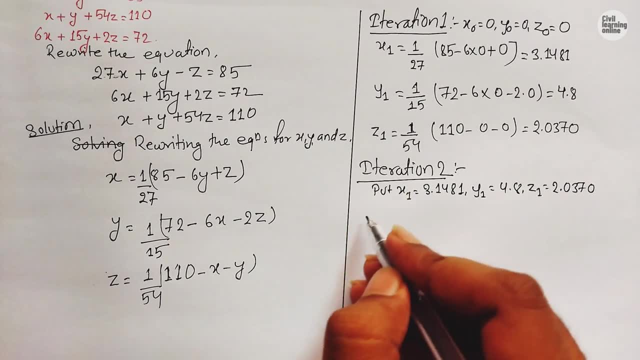 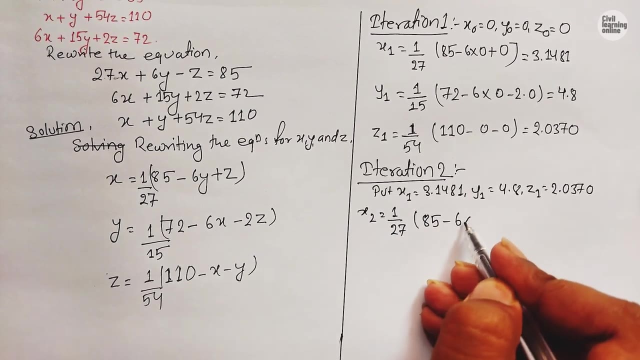 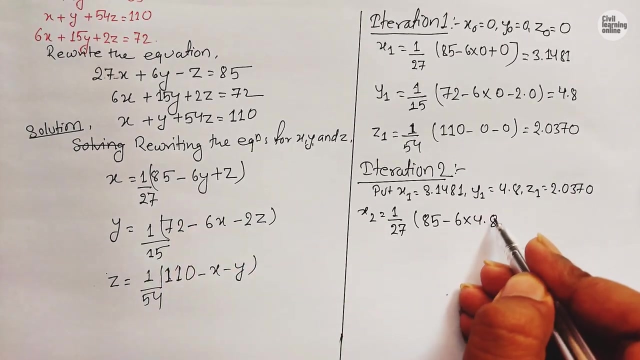 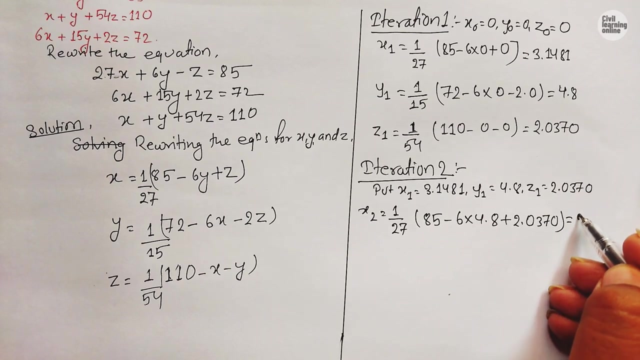 y1 equals to 4.8 and z1 equals to 2.0370. we will have here for iteration 2: x2 equals to 1 upon 27 times 85 minus 6 times x1. in place of y we have to put 4.8 plus 2.0370, so we will get x2 equals to. 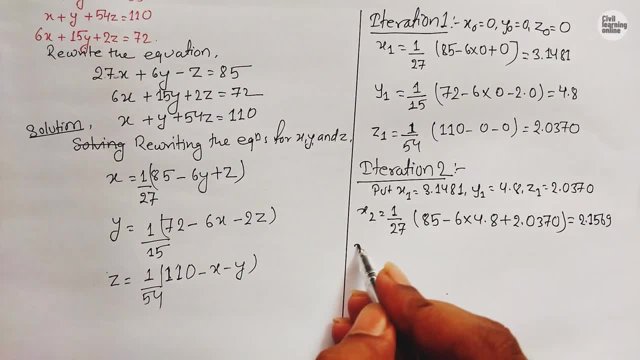 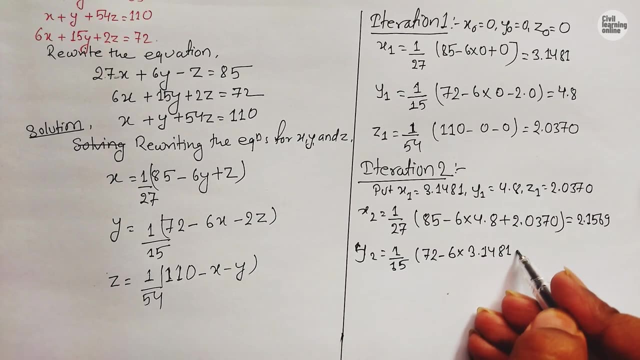 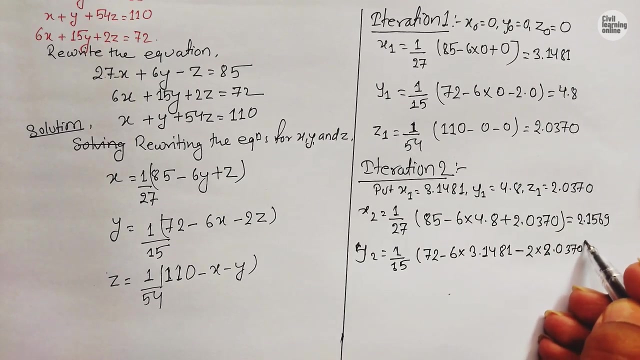 2.1569. similarly, we have y2. y2 equals to 1 upon 15 times 72, minus 6 times 3.1481, minus 2 times 2.0370. so on solving this, we will get the value of y2 equals to. 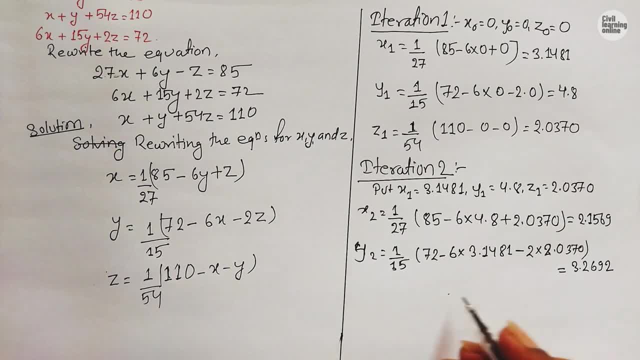 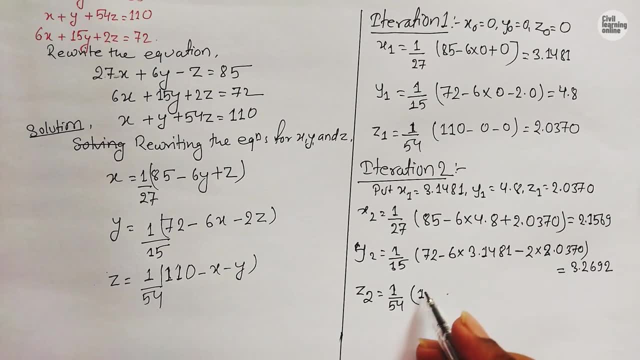 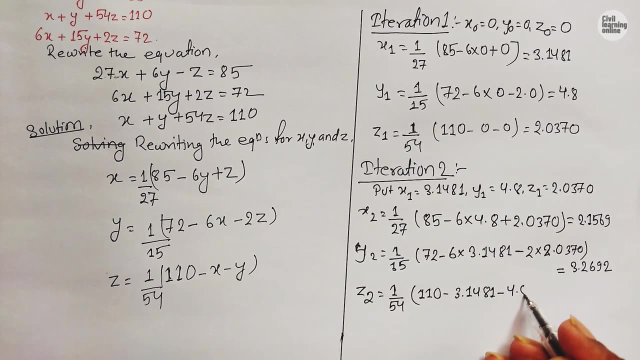 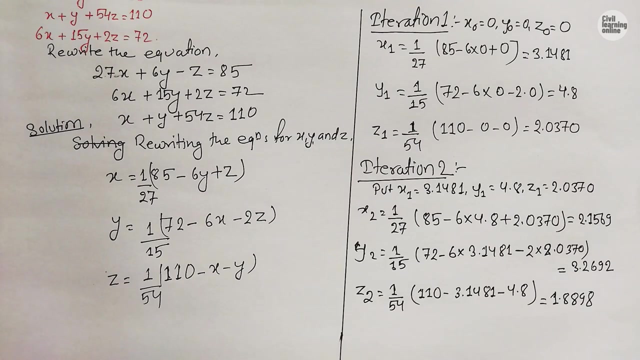 3.27 692. similarly we have z2 equals to 1 upon 54 times 110 minus 3.1481 minus 4.8, we will get z2 equals to 1.8898. now we will do the third iteration, so we will have here x3 equals. 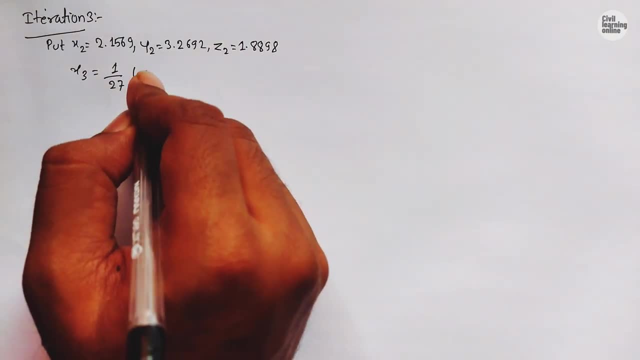 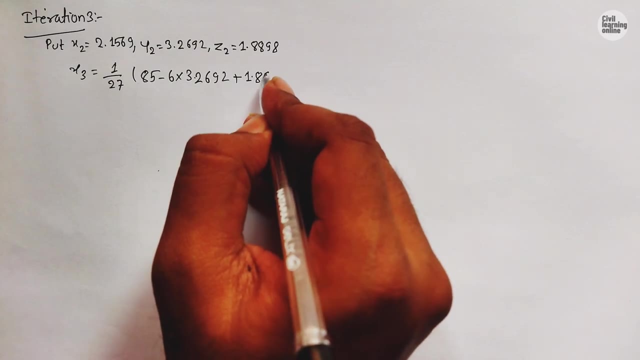 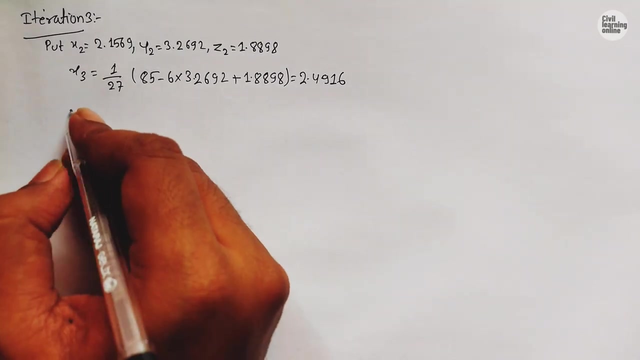 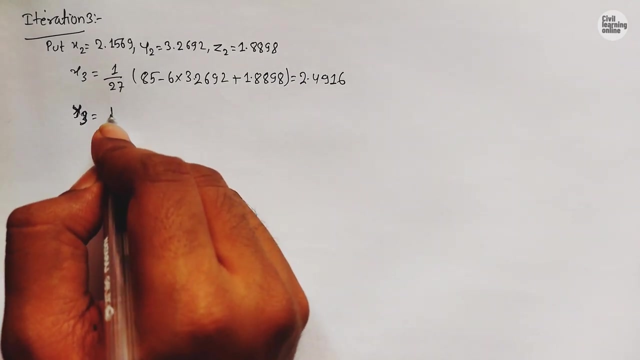 to 1 upon 727 times 85, minus 6 times 3.2692, plus 1.8898, we will get 2.4916. similarly, we have x4. someone say y2, y3, sorry, y3 equals to 1 by 15 times 72 minus 6 times 2.158, we will get 2.4916. and 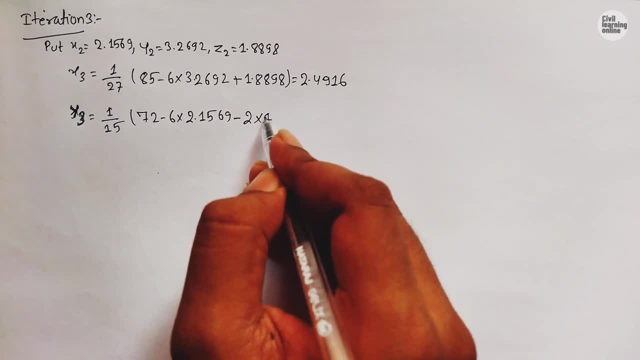 569 minus 2 times 3.4874, minus 1.8はい más 15 Germany miles minus two times 1.8898. so we serving you get 3.6852. so we will get x 1 ele bunny eliminated 0.38.. 159 times. how many timeszed 3.p. expand v2 to x1 by 74 times 1.58했습니다еч9.. x2, similarly z3, equals to 1 by 54ifex150-4 pointed 1.291569 minus 3.2692we will get 1. seek. 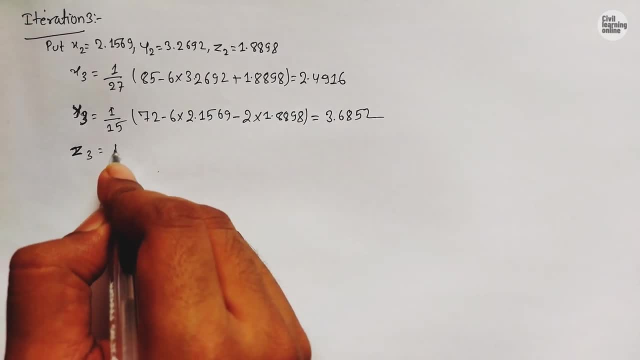 269 minus 3.2692, we will get x 1. trip by one hundred ten minus two: 1569: 12 solution: x 2 times 1000 minus 3.8698: Railway LOOK, we will have x 1 equals to 1. twitter. 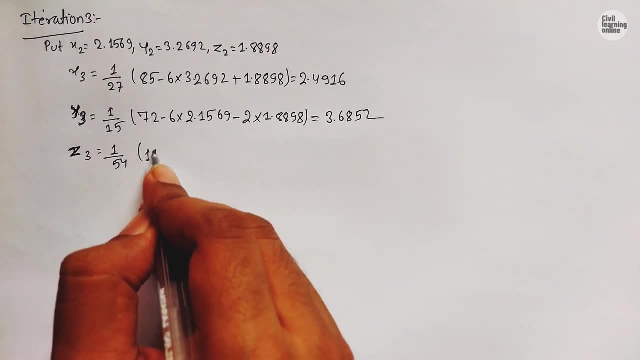 ingress, first step to the environment. so we need to find cand classroomsMарck on 구 created those columns and how can we apply it? and 20 demolish these? class 0שיםight business, 3 coutumars. data and Analytical. 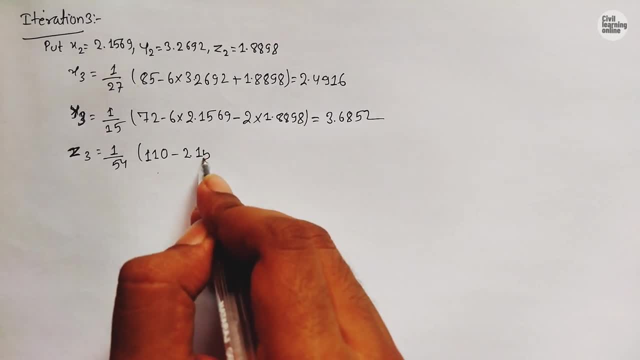 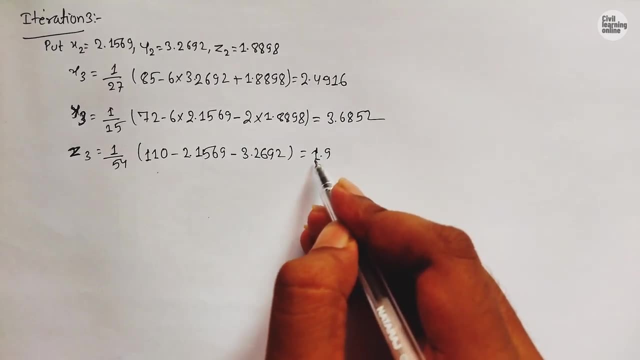 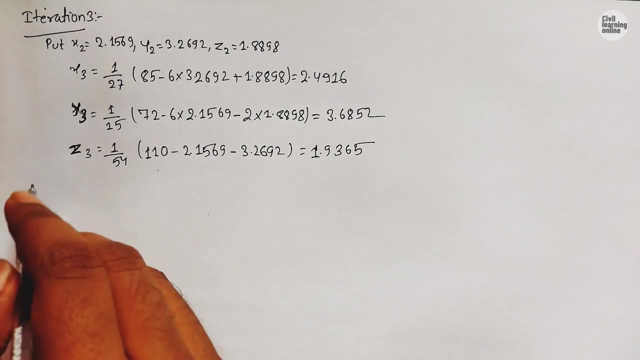 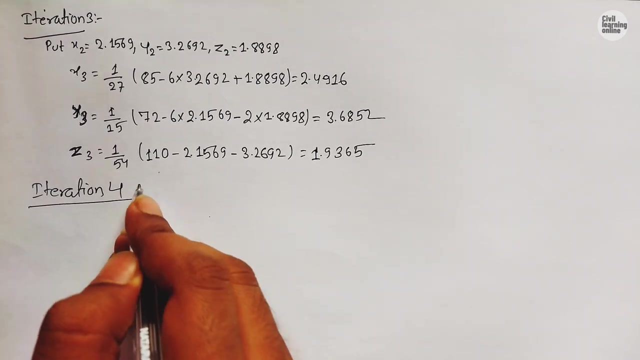 10 minus 2.1569 minus 3.2692, we will get 1.9365. okay for iteration 4. now for iteration 4. for iteration 4, what we will do? see here: we are not getting the value close. we will stop doing. 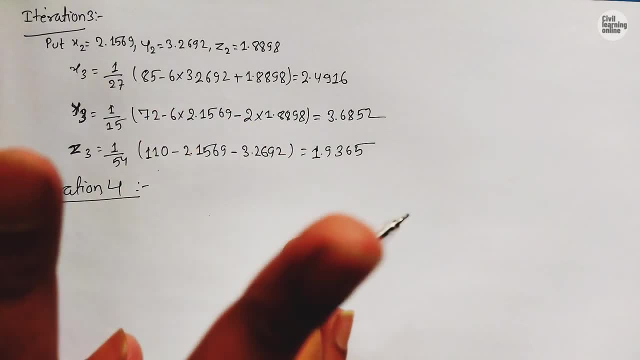 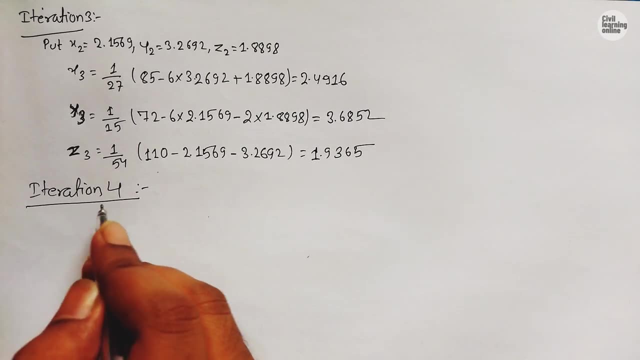 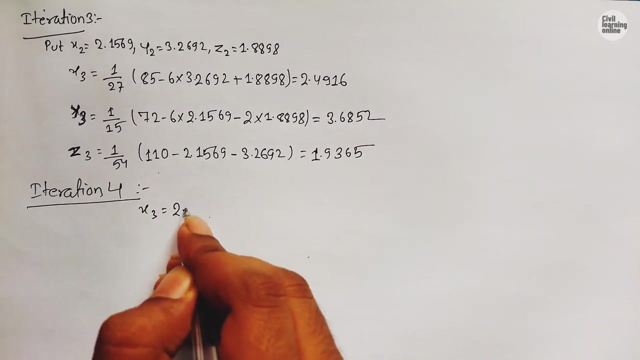 iteration. when we when the two iteration in two iteration, we will get the same value of x, y and z. we have not got yet now, so we will do for iteration 4. for iteration 4 we will use this value, this value of x3, y3 and z3. so we have here: x3 equals to 2.4916, y3 equals to 3.685. 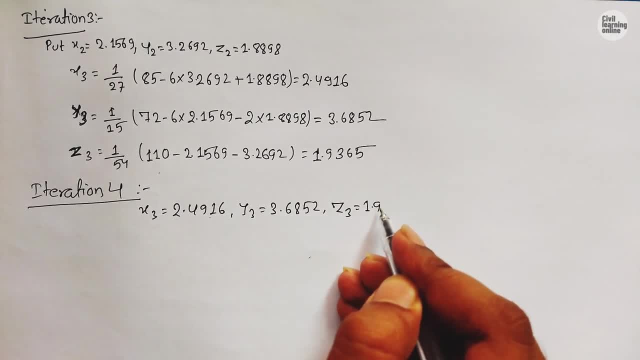 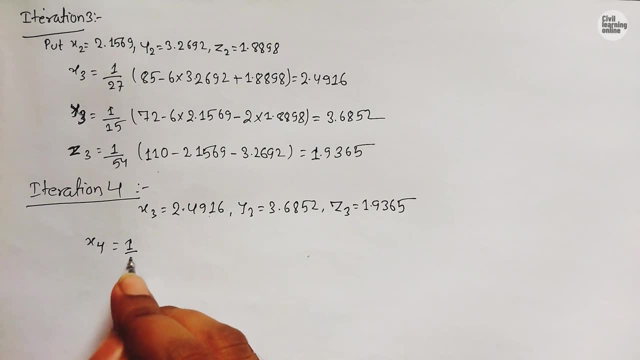 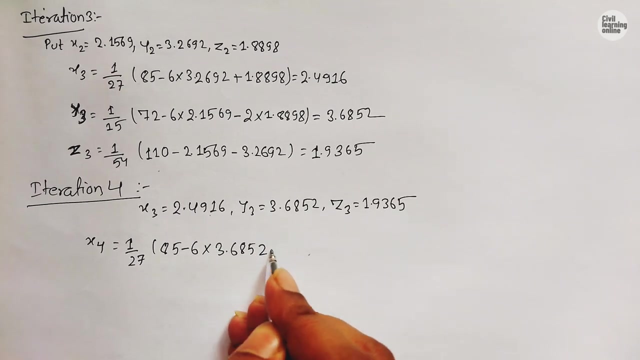 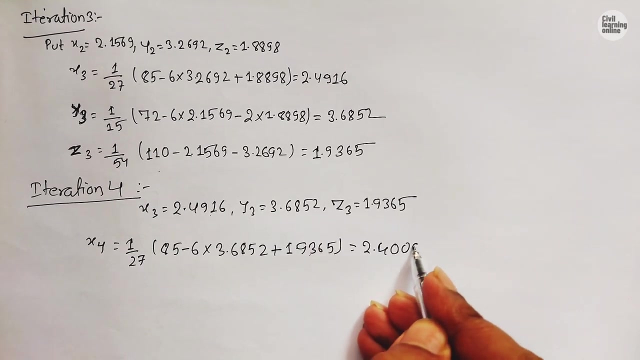 2 and z3 equals to 1.9365. so we have here: x4 equals to 1 upon 27 times 85, minus 6 times 3.6852 plus 1.9365, we will get 2.4009. similarly y4 and z4. 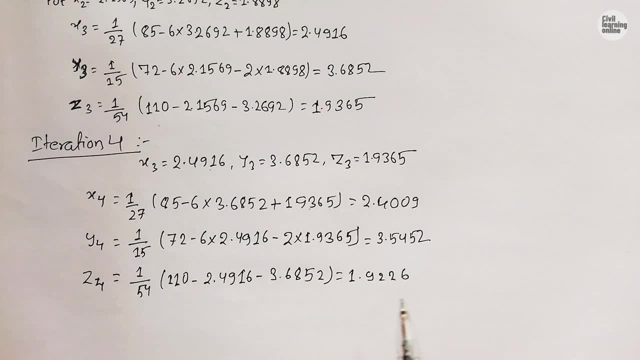 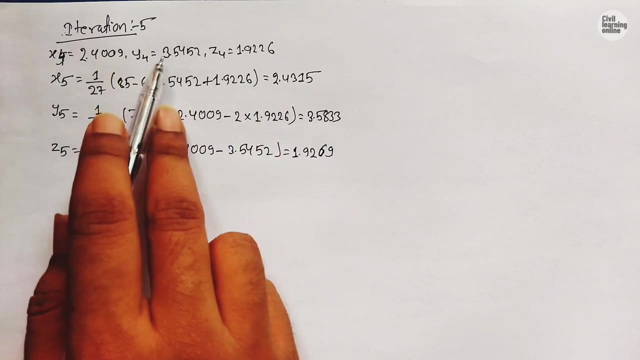 so this is for iteration 4. we have still not got the value similar in iteration 3 and iteration 4, so we will move for iteration 5 now. so here we have. we have done iteration 5. in iteration 5 also the value is varying of x, y and z. so again we will do for. 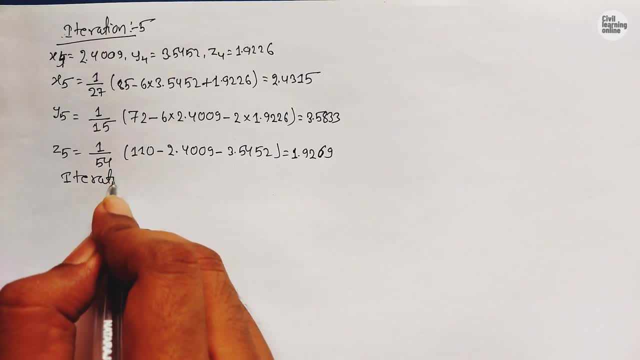 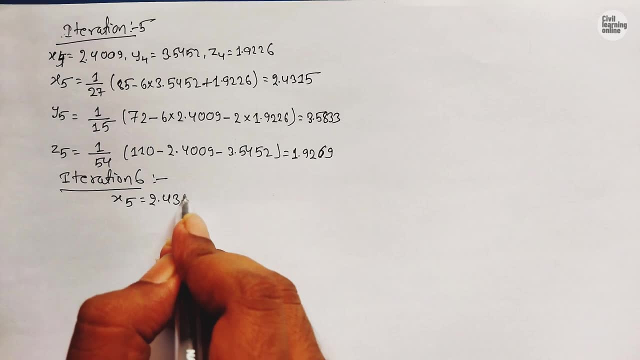 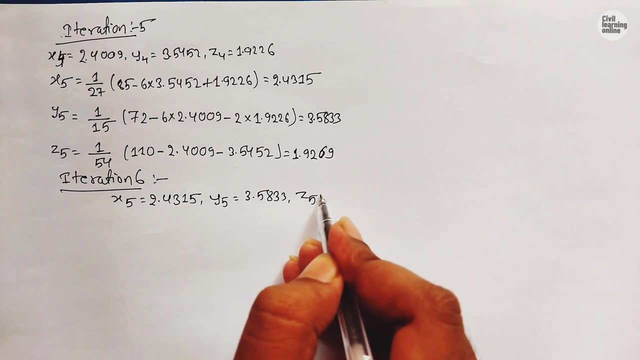 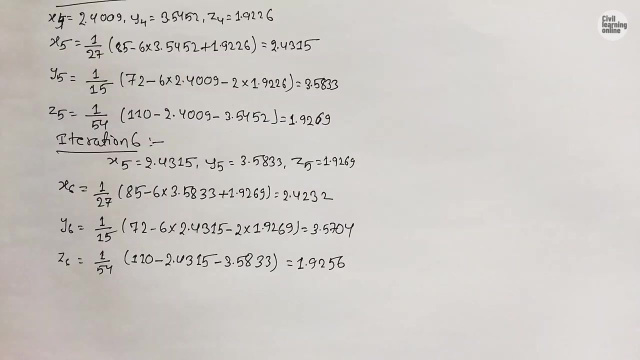 iteration 6. in iteration 6 again we will use x: 5 equals to 2.4315, y5 equals to 3.5833 and z5 equals to 1.9269. so we will have here x6 equals to. so here again in iteration 6, we are getting the values, which is not 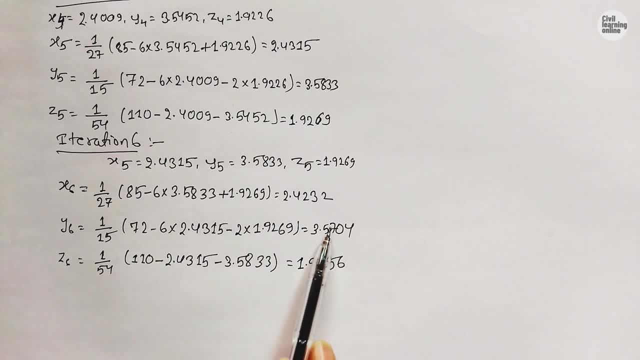 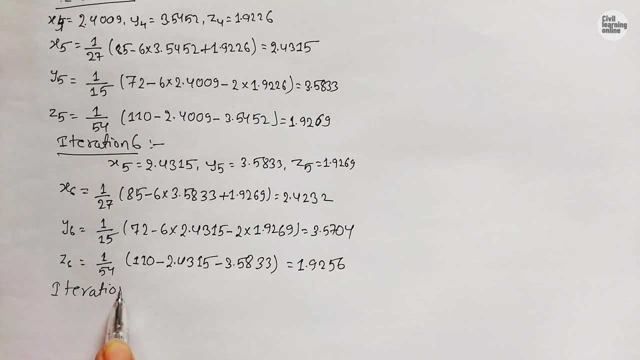 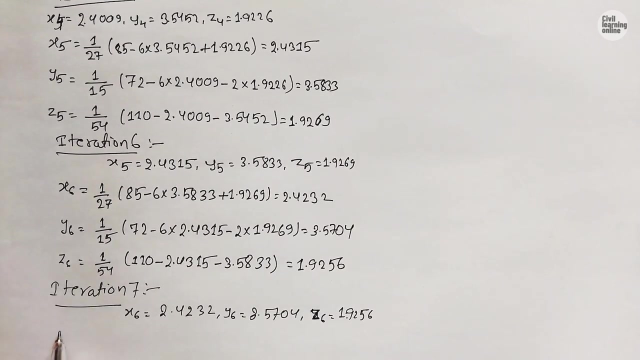 matching with the values of iteration 5. it is varying. so again we will do iteration 7 and iteration 7. we will use: x6 equals to 2.4232, y6 equals to 3.5704 and y6, z6 and z6 equals to 1.9256. so we have x7 equals to, x7 equals to. 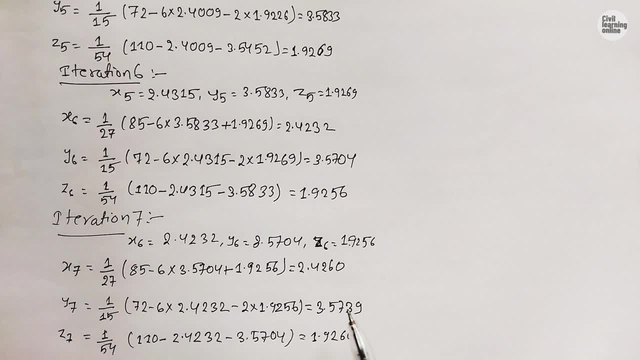 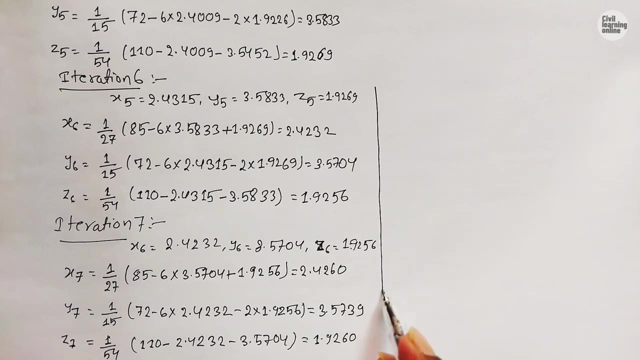 Here the value is varying little by little. means in iteration 8, we may get the value similar to means we may get exact value in iteration 8.. So let us check for iteration 8 now. So I am going to use this portion for iteration 8.. 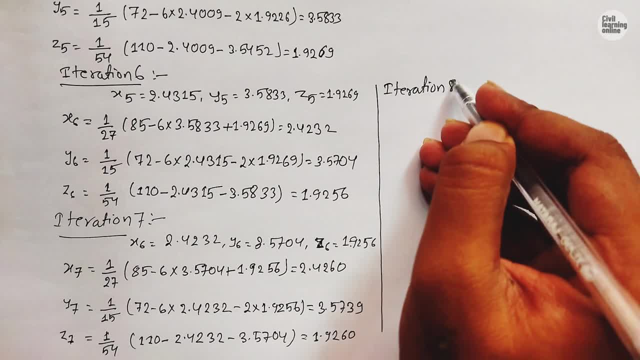 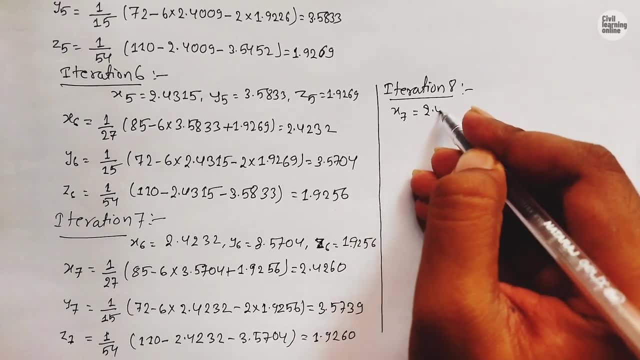 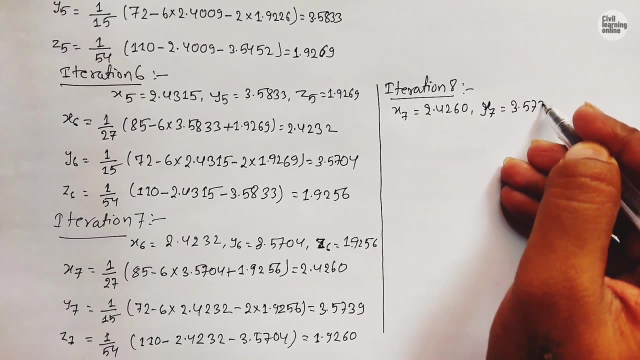 See here iteration 8,. for iteration 8, we will use the value, what we have got in iteration 7, that is, X7 equals to 2.4260, Y7 equals to 3.5739 and Z7 equals to 1.9260. 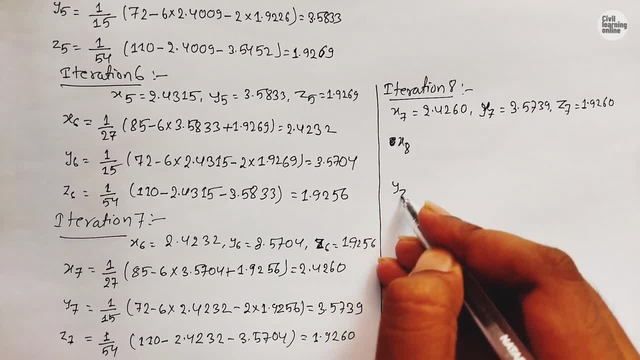 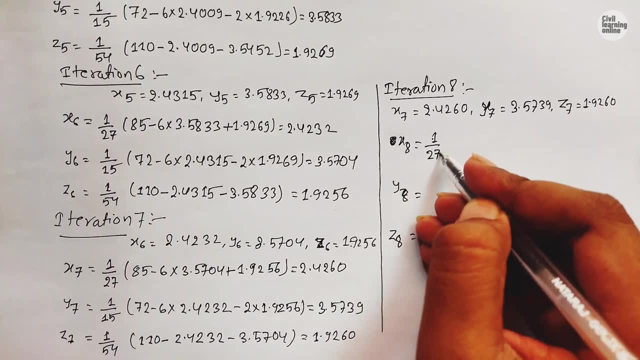 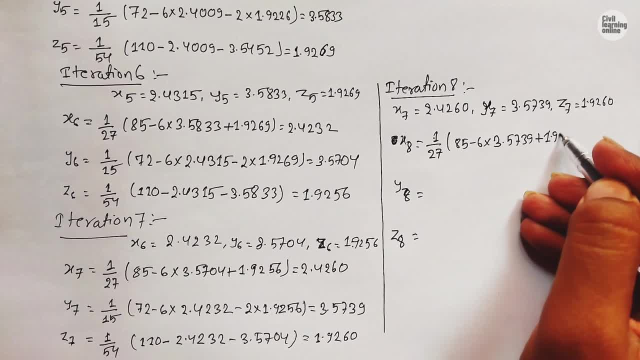 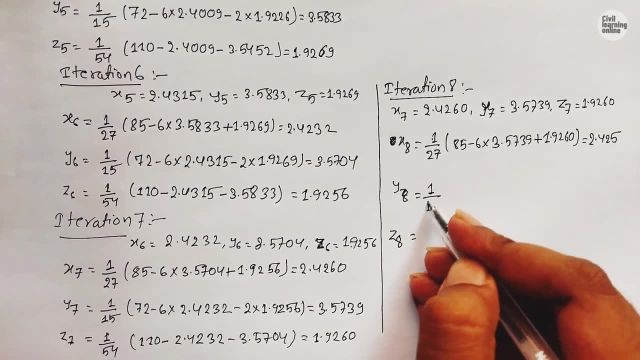 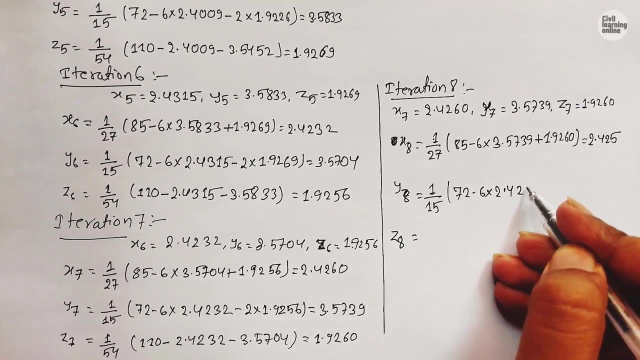 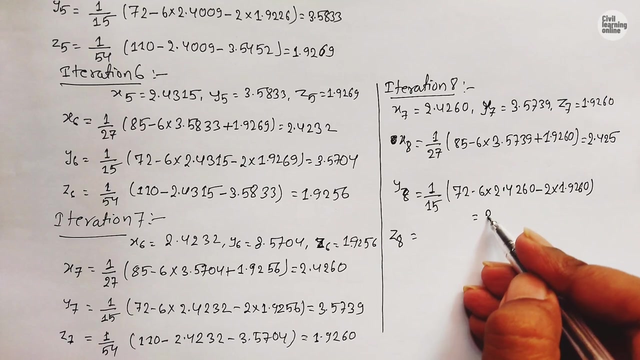 5739 plus 1.9260, we will get 2.425, again, 1 upon 15 times 72, minus 6 times 2.4260, minus 2 times 1.9260.. We will get here 3.5728.. 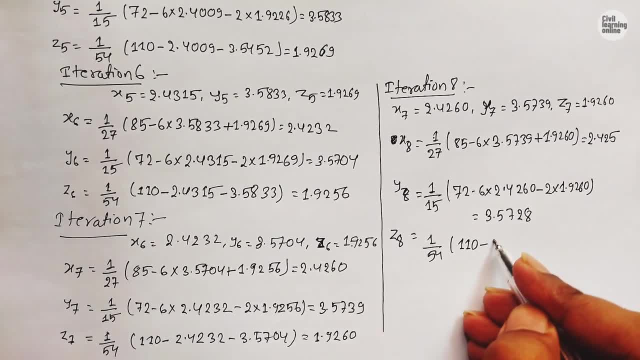 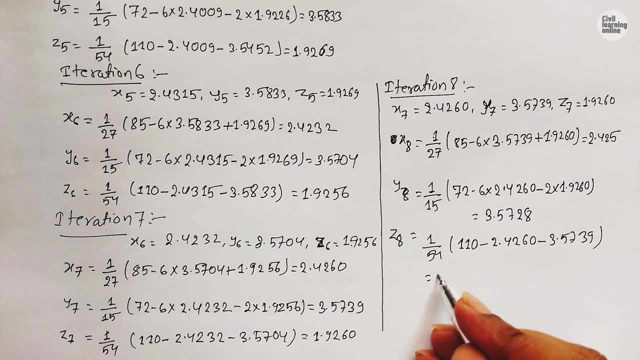 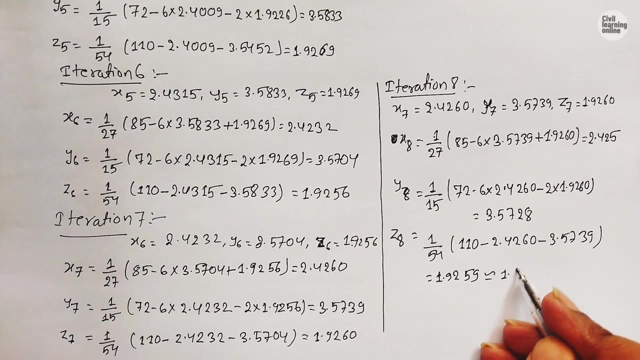 54 times 110 minus 2.4260, minus 3.5739. on solving this, we will get z z 8 equals to 1.9259, which is, which will be approximately equals to 1.9260. on doing round off means we have got the value. 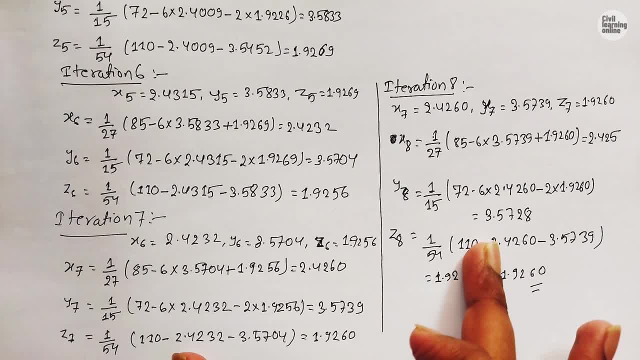 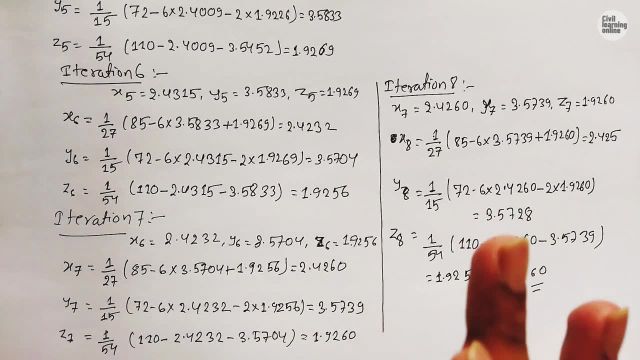 of iteration 7 and 8, exact as it is. so this is the end of this numerical. i hope you enjoyed this lecture and learned how to do jacobis iteration method. see you in the next video. till then, stay safe and take care of yourself and guys, if you are enjoying the content on civil learning online, 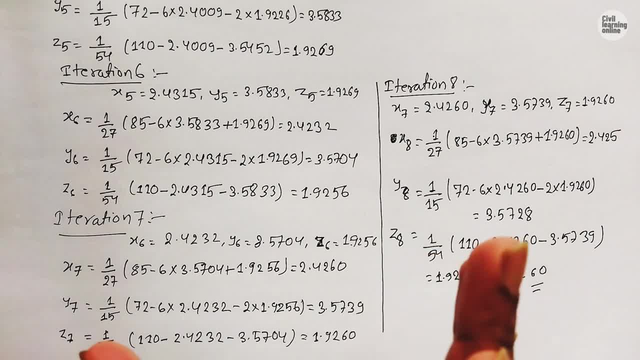 channel, then do like this video. suggest this video channel with your friends. share this video with your friend and see you bye.